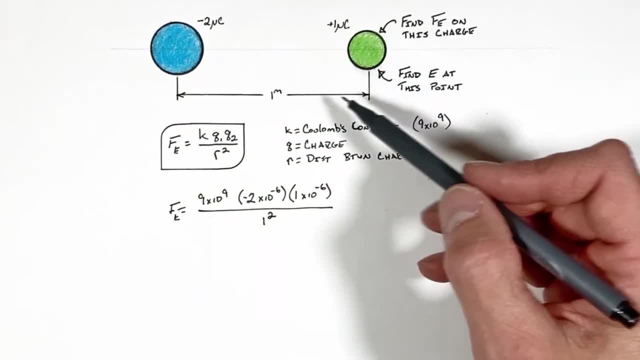 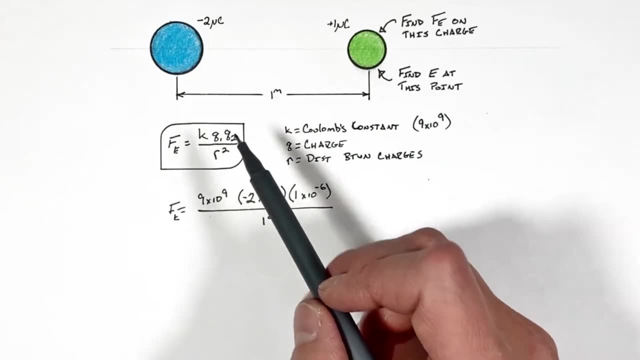 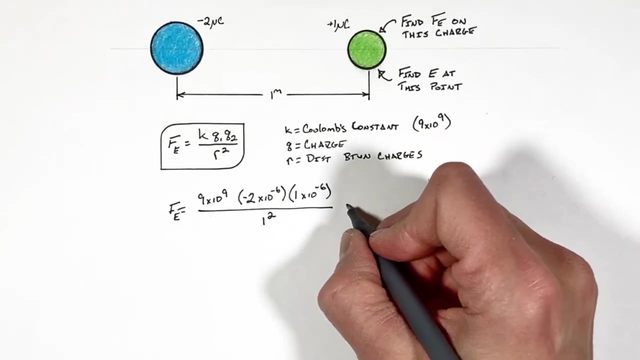 or not. they need to take this distance and divide it by 2, like you would in looking at the diameter versus radius of a circle. and that's not true. it's r, however misleading it is, is truly the center to center distance of these two charges charges. now, working this out, we find the electric force is negative, point zero. 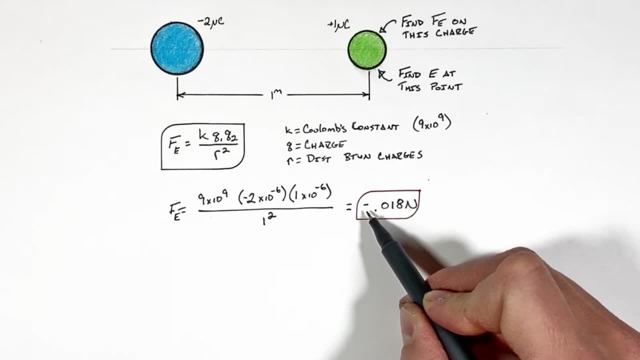 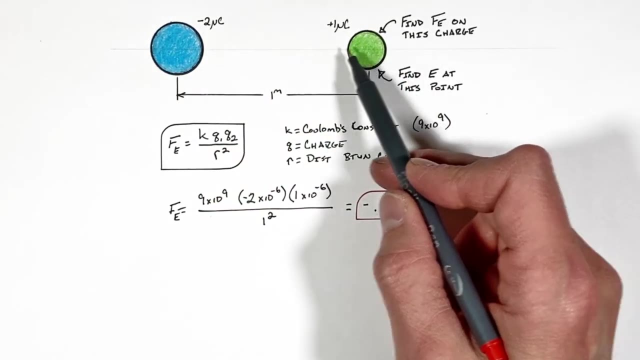 one, eight Newton's. now we need to talk about the meaning of this negative sign right here. see, this negative doesn't have anything to do with whether the force is left or right. what this negative is telling us is that the force between these two charges is actually causing them to be pulled towards each. 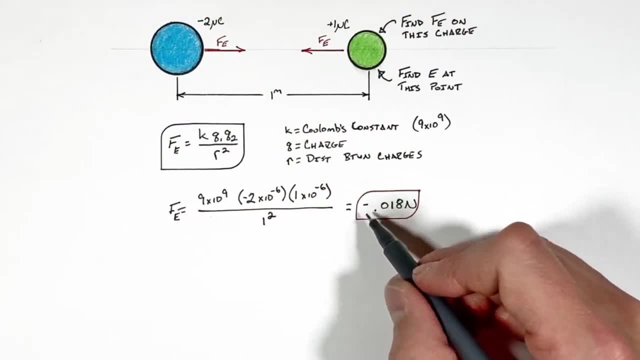 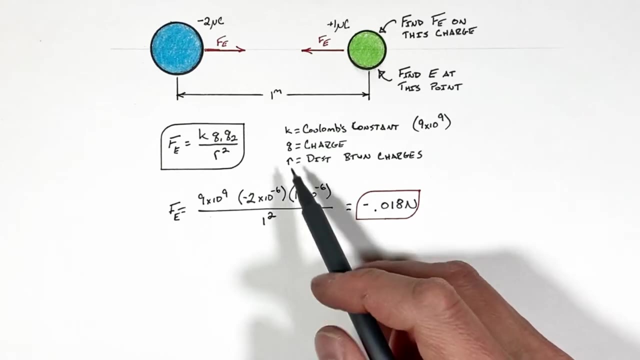 other. if this result had come out positive, that would mean the two forces were actually pushing away or repelling each other. and if you look at where this negative came from, it exists because these two charges had opposite signs. ultimately, going back to the idea: the opposite charges attract each other and 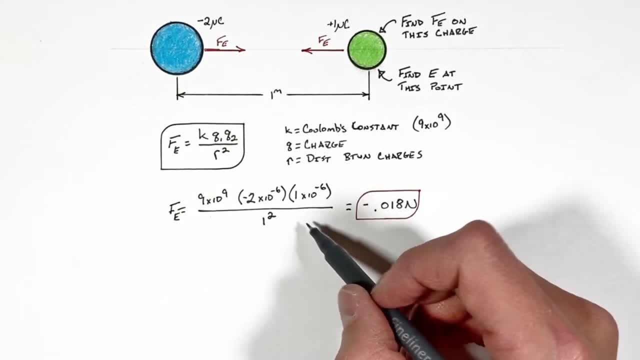 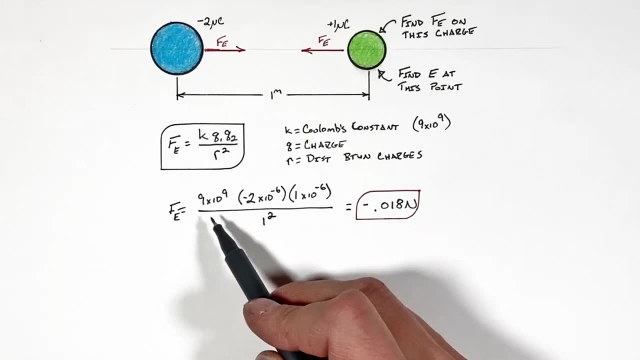 similar charges repel each other. if we had two charges with the same sign here, this electric force would have come out positive you. so, now that we know the electric force, we can. so, now that we've solved for this electric force, we can now turn our attention to solving for the electric. 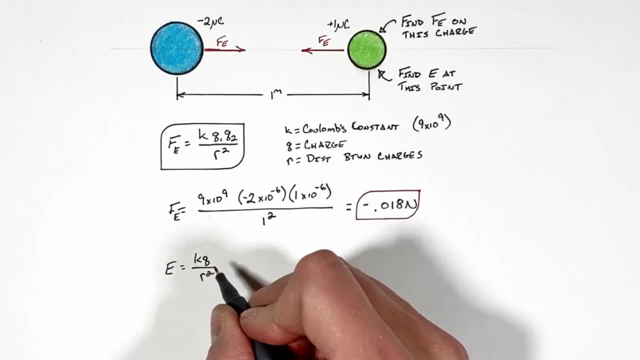 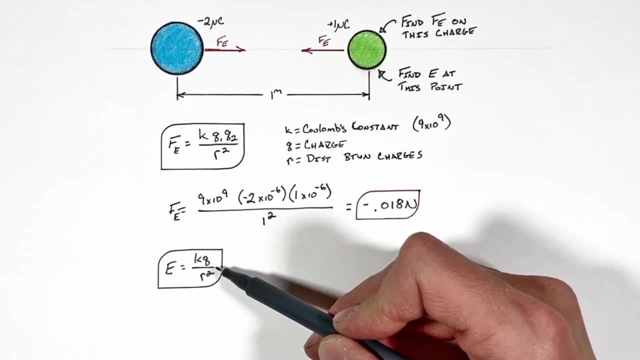 field. at this point the equation for electric field looks an awful lot like coulomb's law, except it only involves a single charge. so the question comes up: if we're trying to solve for the electric field at this point, which charge do we need to use? now you'll remember we're solving for the electric field at 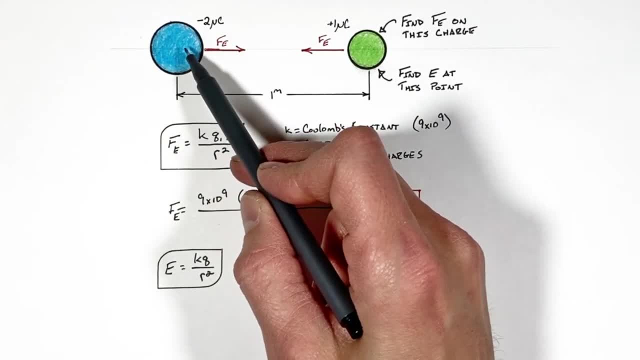 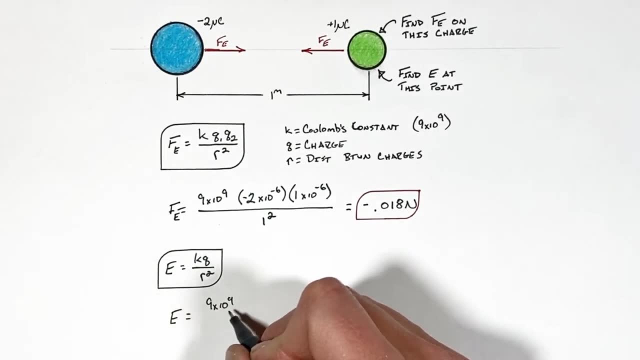 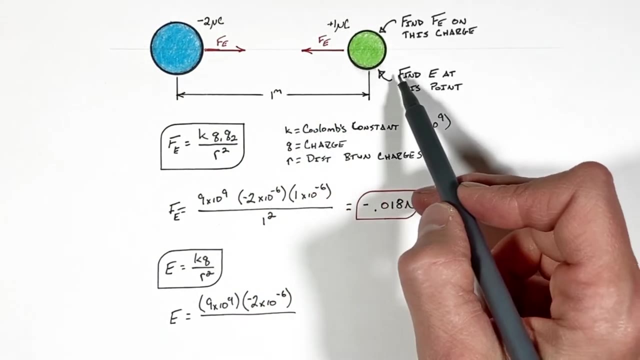 this point as a result of this charge. so we're going to use the magnitude of this charge in our equation for electric field, again using coulombs constant multiplied by the magnitude of this charge over the distance between this point and our two micro coulomb. 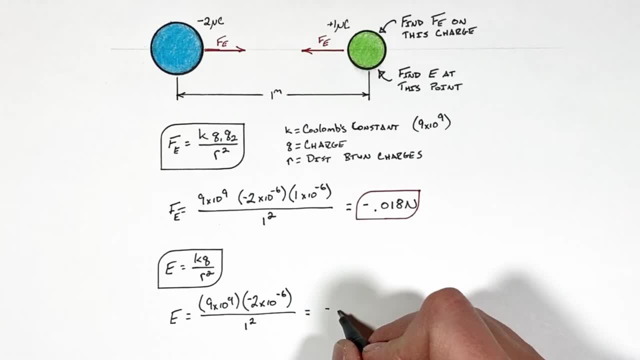 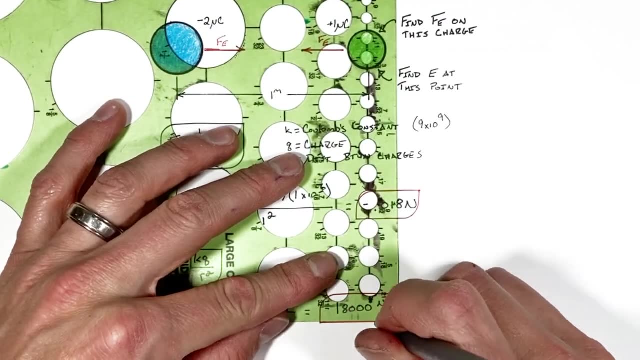 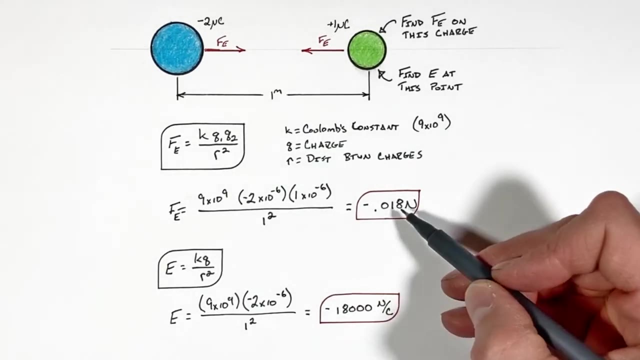 charge and this gives an electric field of negative 18,000 Newtons per coulomb and much. like we did up here, let's talk about what this negative for electric field means. see, this negative, just like before, isn't telling us about whether or not the electric field is.